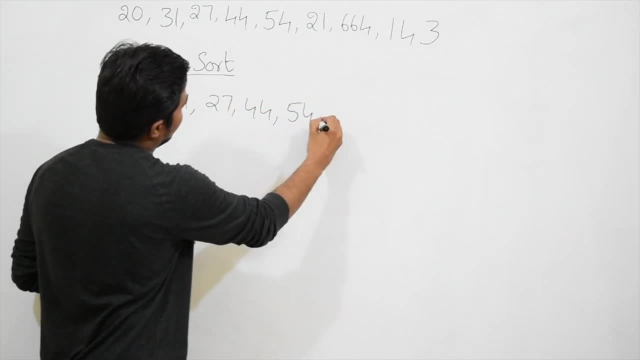 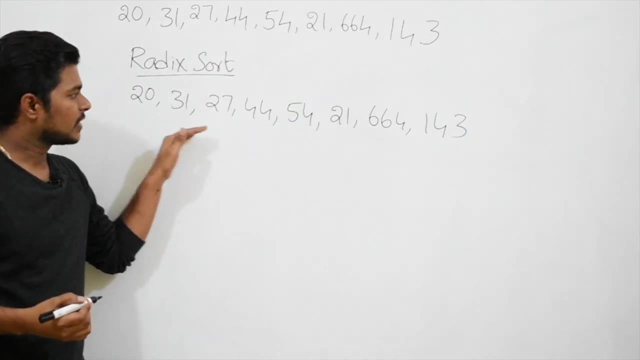 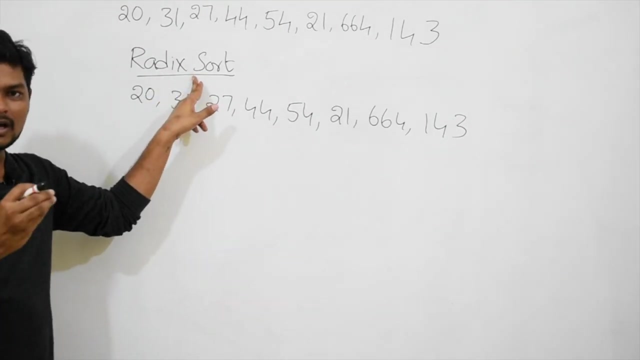 27,, 44,, 54,, 21,, 64, 143.. So these are the given numbers which we need to sort. Now. this Radix Sort Algorithm can be performed based on the Counting Sort. Okay, This is performed basing on Counting Sort Mechanism. 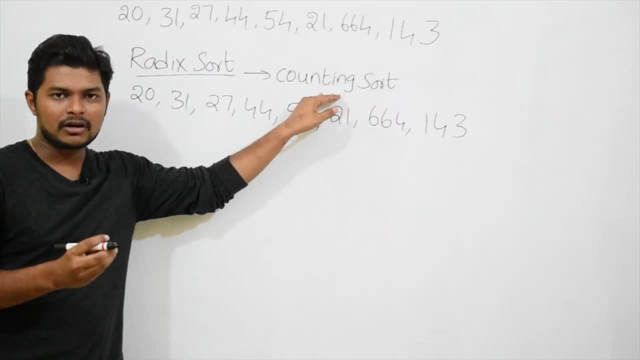 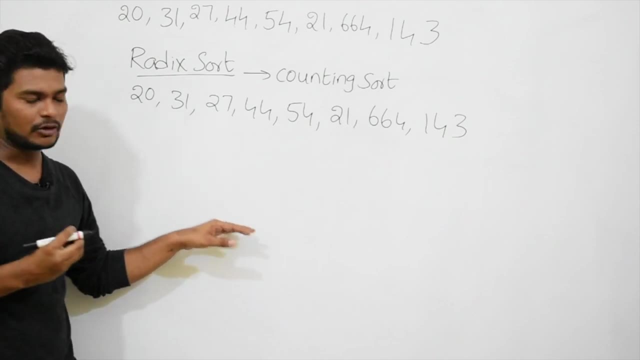 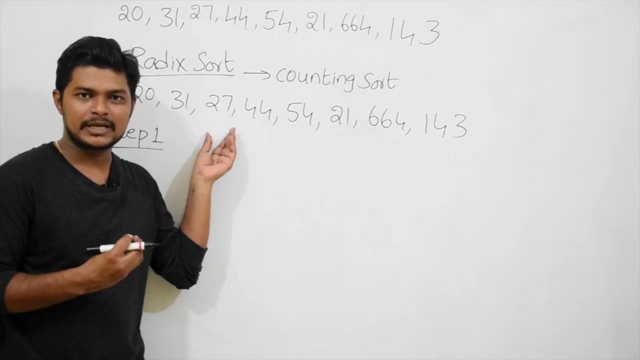 And as we know that Counting Sort is a stable sorting algorithm, the same stable sort will apply here also. Okay, this can be performed in step by step, which we are going to see now. Okay, in step one. Now, what we are going to do in step one is: you take the given numbers. 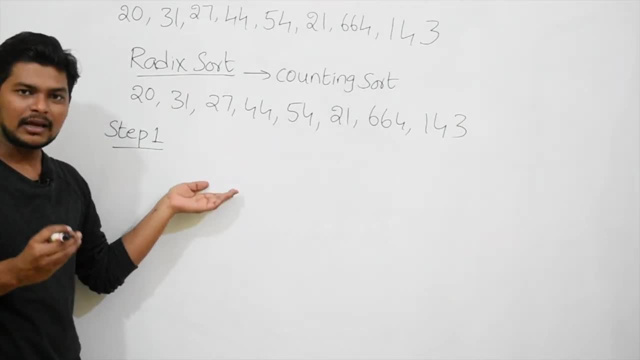 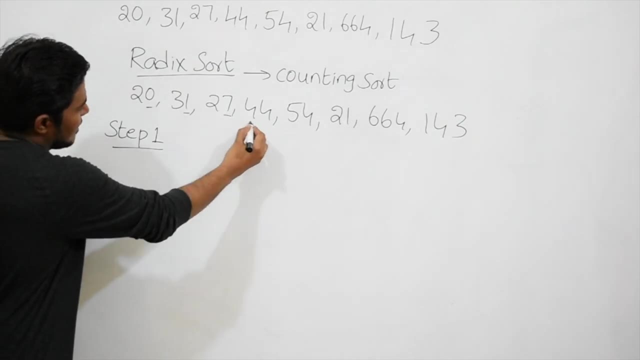 you go to the last digit And sort according to the basing on last digit. Now, here this is a two digit number. Last digit is zero. Here last digit is 1, 7,, 4, 4,, 1, 4 and 3.. 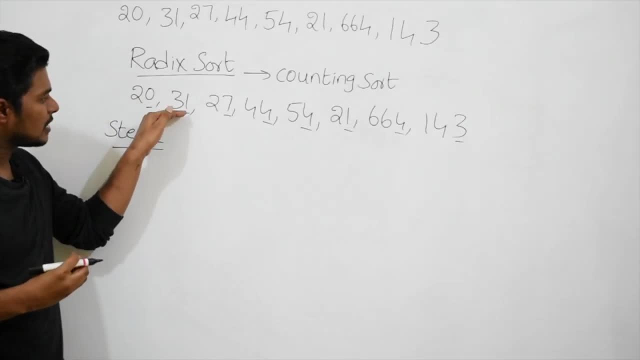 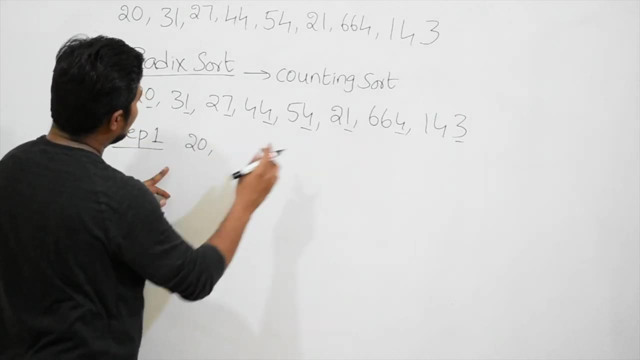 Now, in step one, what we are going to do is sort based on the last digit. Okay, Now here, zero will come first, So write 0, 20, then any ending with 0, no Ending with 1 is 31.. 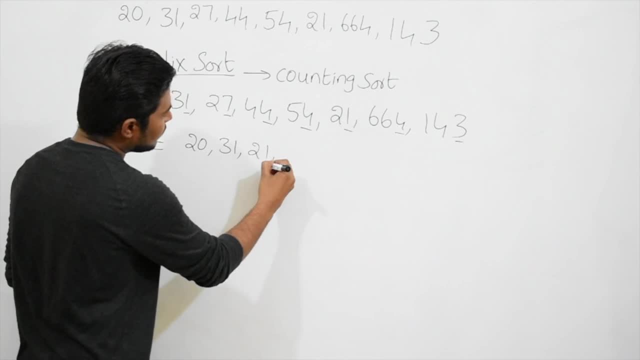 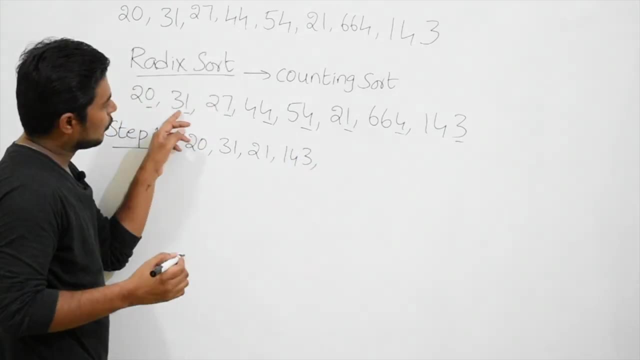 Any ending with 1, yeah, 21 is there Now, like that. Now ending with 2, none Ending with 3, yeah, 143 is there Now. ending with 4, yeah, 44 is there, 54 is there, 6, 64 is there. 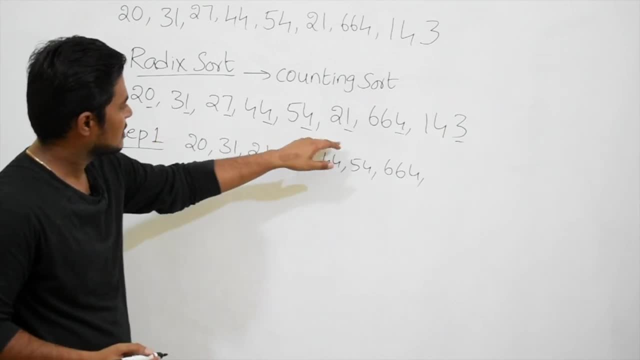 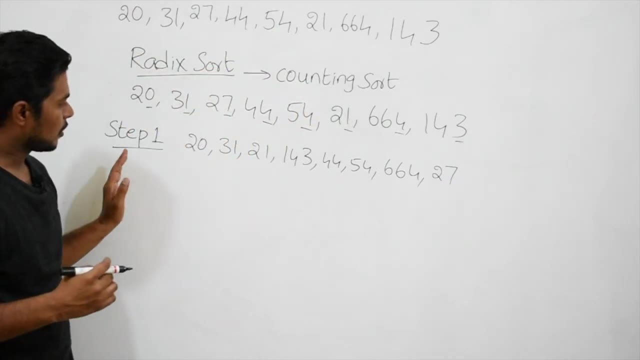 Now ending with 5, nothing Ending with 6, nothing Ending with 7 is 27.. So now we need to count the numbers. Given numbers are n equal to 8.. Now we have to see whether here 8 is there or not: 1,, 2,, 3,, 4,, 5,, 6,, 7,, 8.. 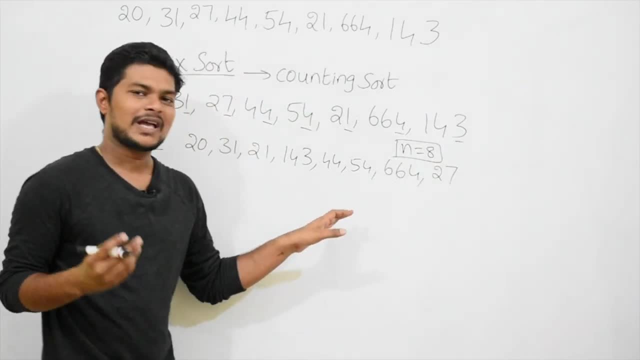 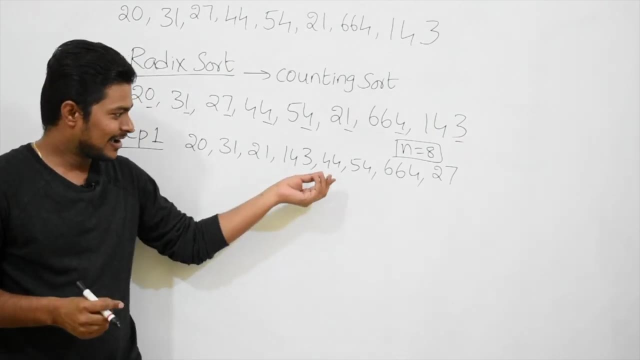 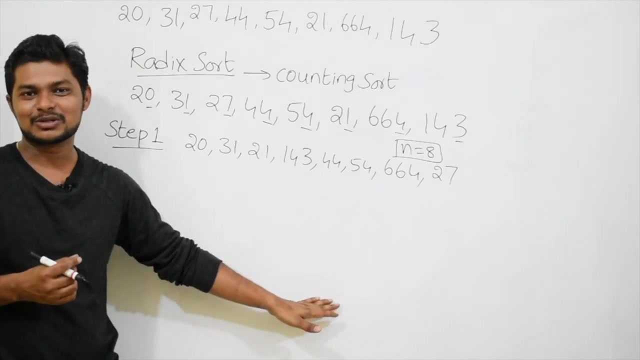 n equal to 8.. There are total 8 numbers. I am counting because maybe we will miss some numbers In the exam also or anywhere. when you are working on a paper, always make a count of numbers, Because if you miss one step, one number also, the complete algorithm goes wrong. 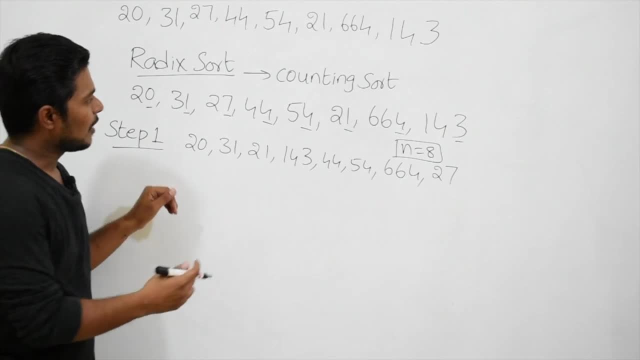 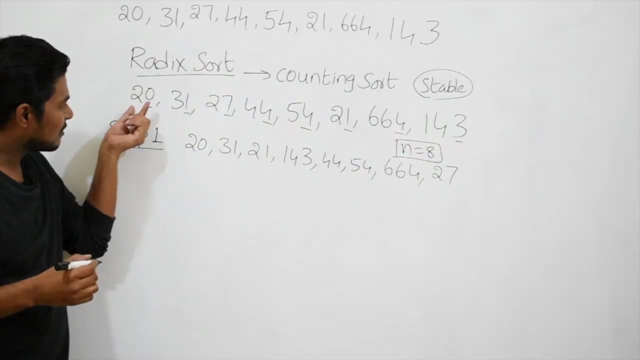 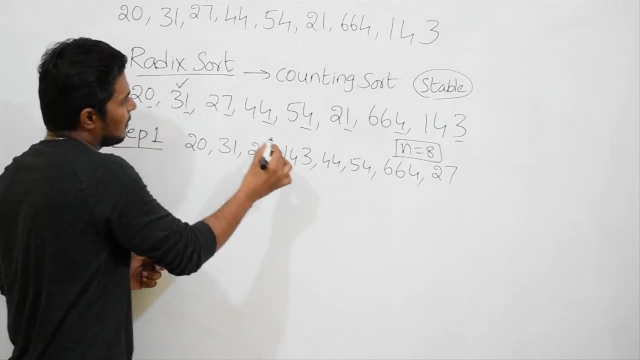 Okay, This is step one completed. Now I said counting sort is a stable sorting algorithm. What do you mean by stable sorting algorithm is, if you observe clearly here, ending with 0, only one number is there. We have written that Ending with 1, two numbers are there: 31 is one number, 21 is another number. 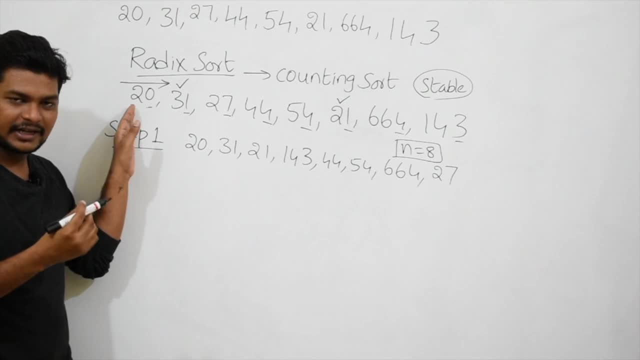 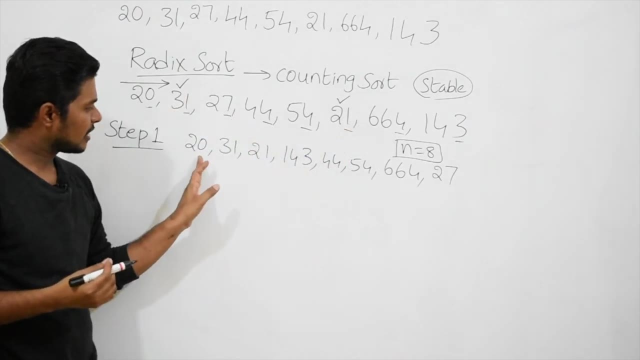 So when we are accessing number wise index, wise 31 comes first, So here also 31 comes first. 31 after 21 came, So 31 after 21 came. Likewise 44, 54,, 664.. Here also same order will be there. 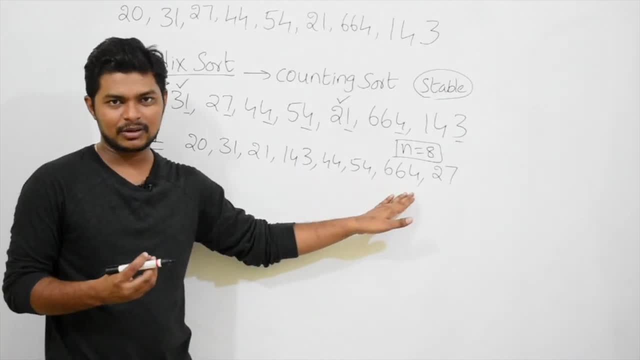 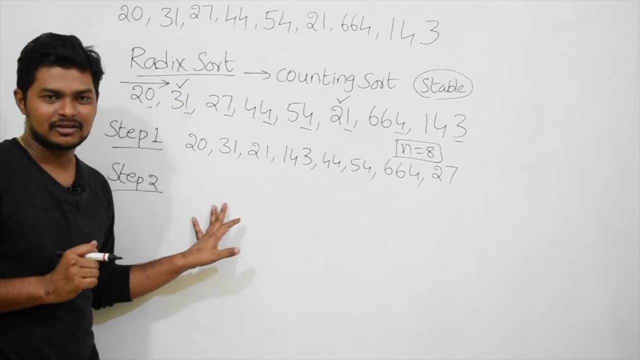 44,, 54,, 664.. This is called stable. Okay, This is called stable. Now, in step 2.. This is stable. This is stable. very, very simple, very, very simple sorting algorithm in step two. what we need to do, we need to take. 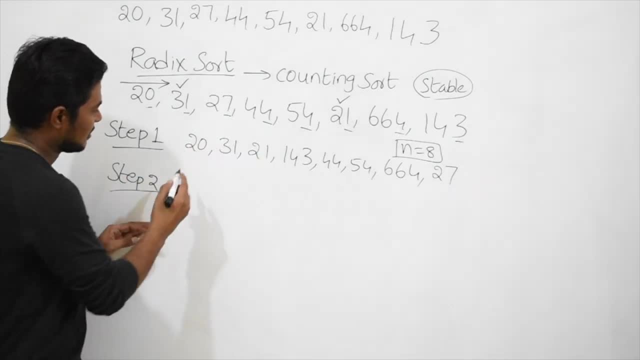 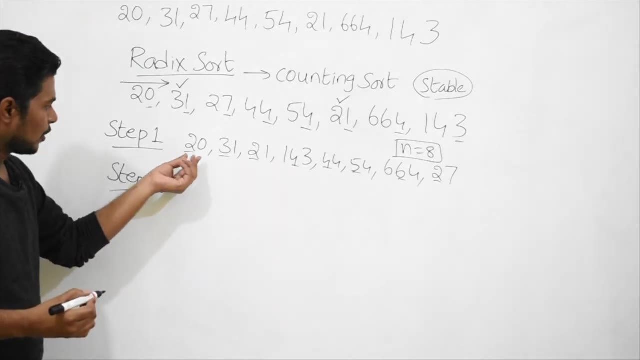 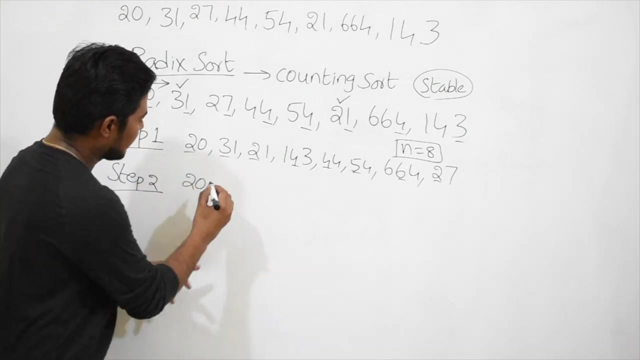 second last digit in the step one. we take a last digit. this is the second last digit: two, three, two, four, four, five, six, two. this is the second last digit. okay, now we need to sort based on second last digit. 20 will be there. is there anything? uh, yeah, 21 is there, then 27 is there? next 3. 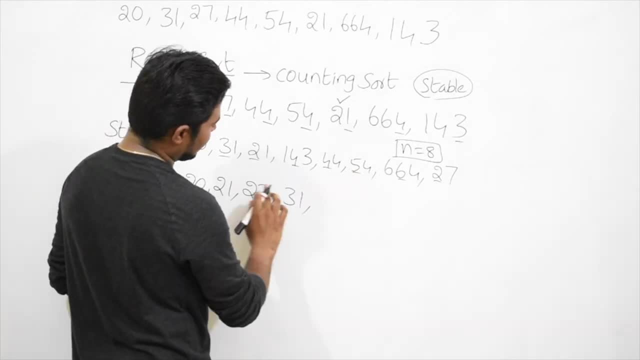 31. is there next 3, 3 nothing next 4. 44. is there next 4, 4 143? sorry, here i need to. this is the mistake. see, i have found out my whole mistake. you also by harry lee. don't, uh, do that here. 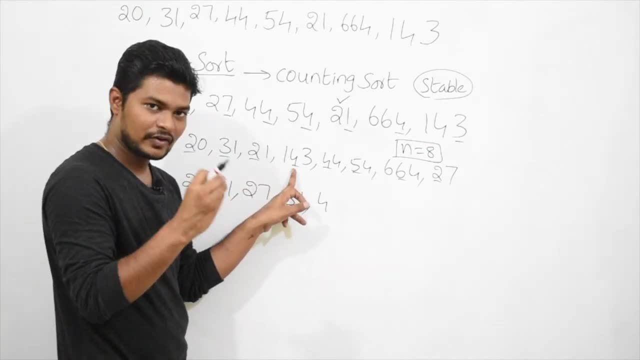 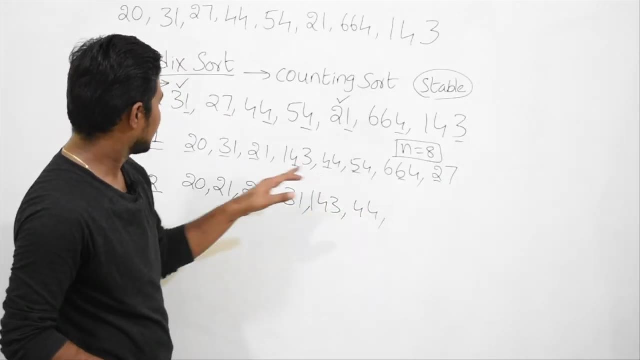 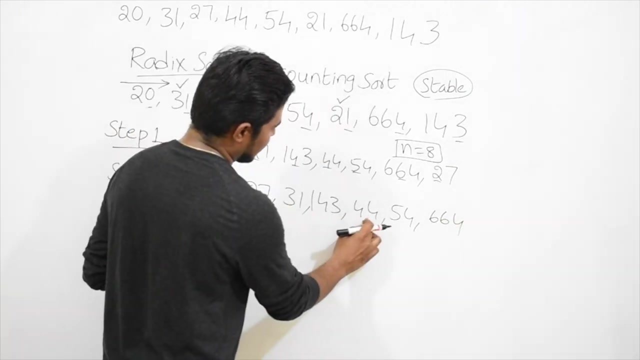 but with the number second digit, 4, 143 comes first, then 44, so right, 143, then 44, then with 4, nothing is there. then with 554, is there, then with 6, 6, 64 is there? count the numbers 1, 2, 3, 4, 5, 6, 7, 8. yeah, now in step 3. this is the final. 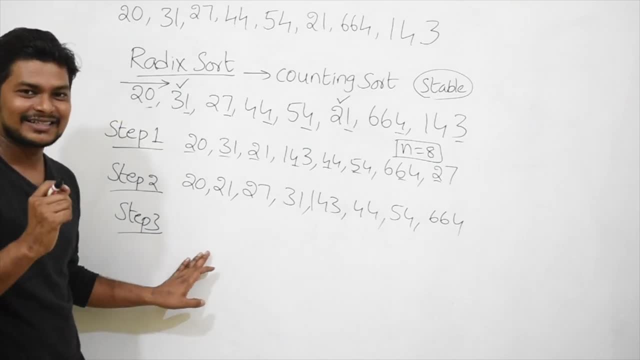 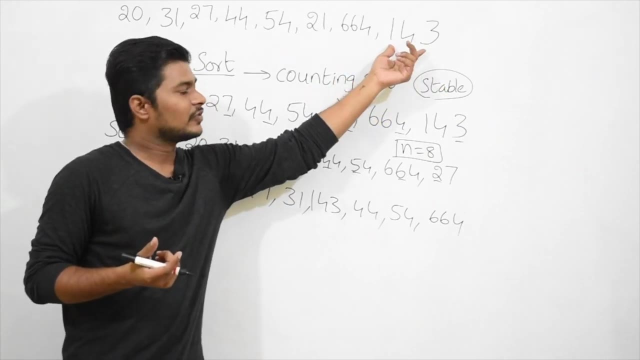 step how i am telling. final step, because this is a shortcut, is there? just remember the range of numbers, with the maximum digits which we can represent is 3, since these are based on. so, within three digit numbers, all the numbers can be represented. so we get the answer in three steps. 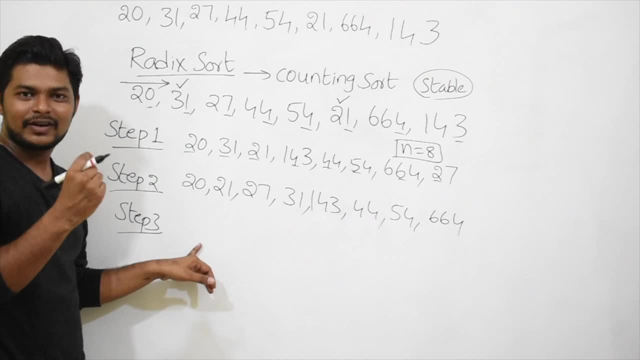 now in step 3, what we need to do is we will sort according to the first number. okay, here, first we will put the number in the third digit. so in childhood we used to represent two digit as three digit number by placing zero in front of that right. here also you have to do the same, so put. 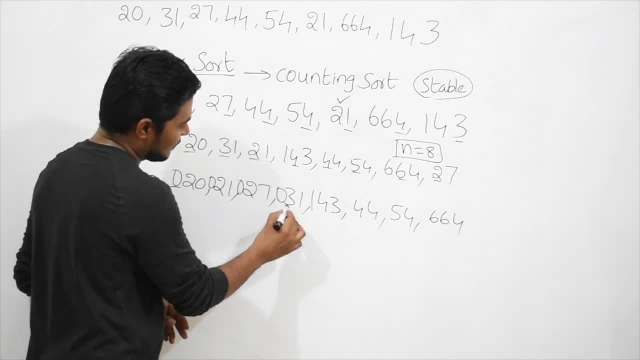 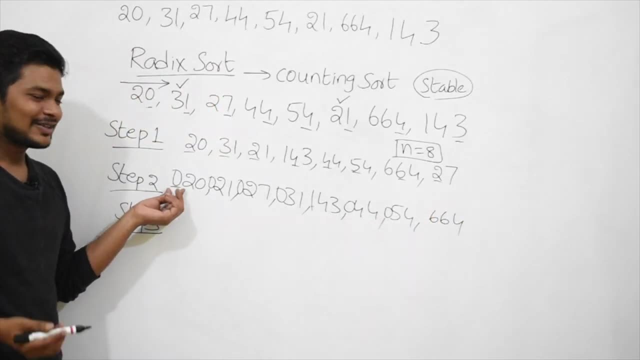 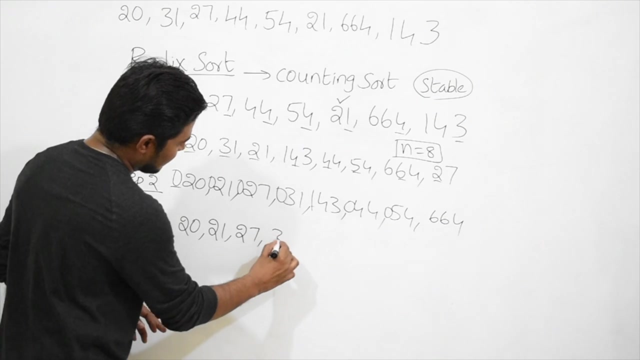 zero 20 becomes zero to zero. likewise zero to one zero two, seven zero three, one, one four, three, zero four, four, zero five, five, five, four, six, six, four. now we are starting. see, starting zero always comes first place, right, so write this: 20, 21, 27, 31. 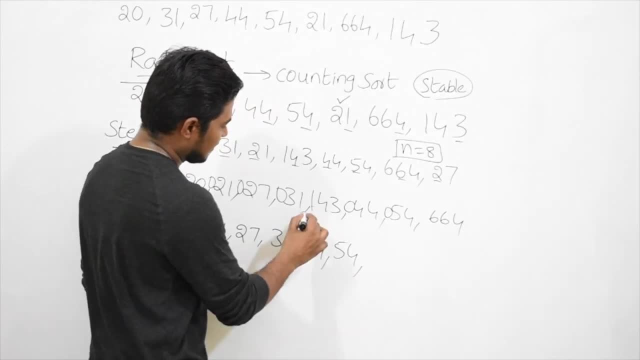 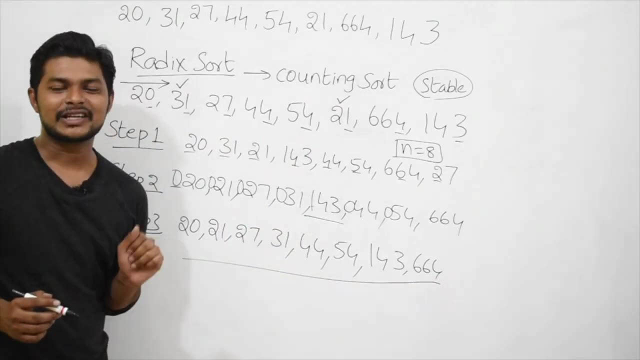 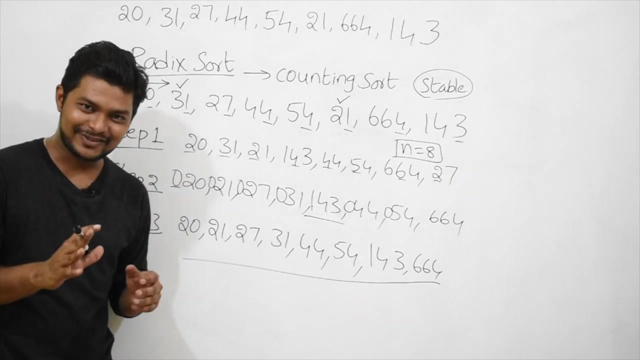 44, 54 after zero. then this comes one, one, four, three, six, six, four. see here we got the sorting algorithm within three steps. see how easy radix algorithm. now, if anyone asks you in your entire lifetime to solve to give like they given some numbers to solve in radix sort, you can solve it. 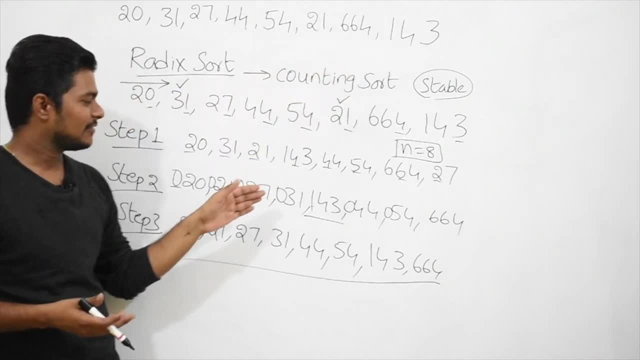 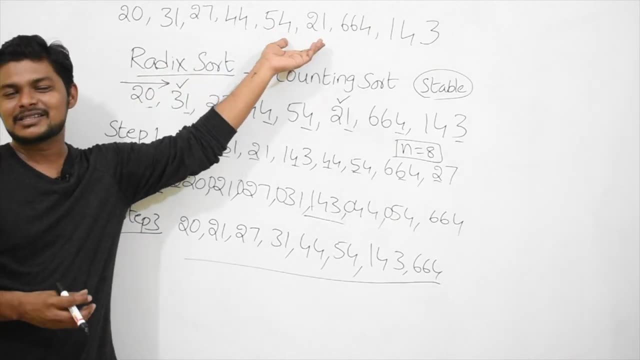 very easily, because if a number is in three digit form it will take three steps. if a number is in three digit form it will take 10 steps. that's it okay. of course, some heavy numbers- if they give like 10 have 20, we can solve. but for sorting some thousands of numbers we need to write a program. 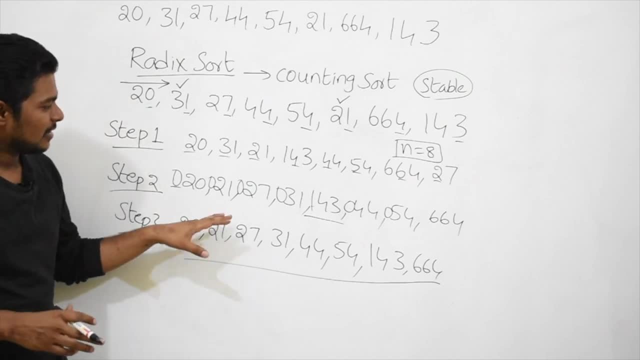 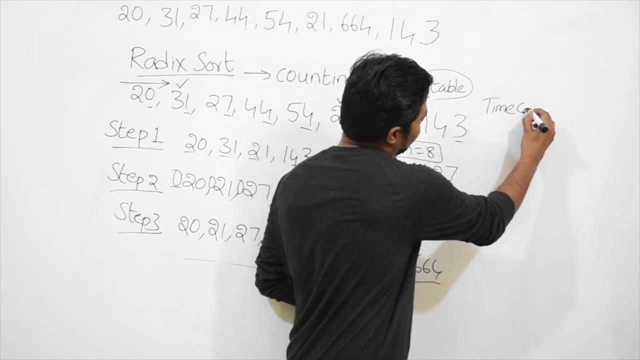 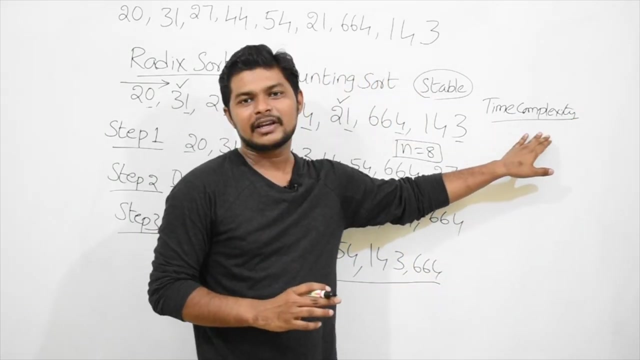 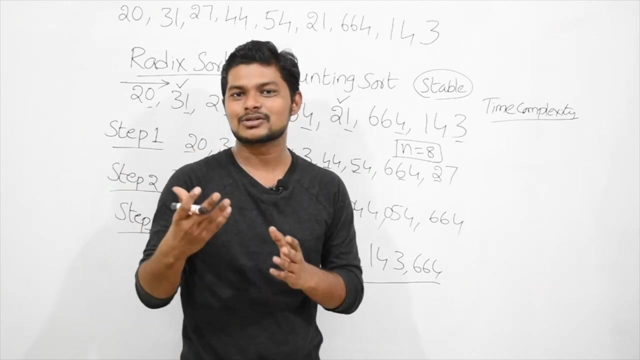 and, believe me, writing a program is also very simple. okay, now we have got sorting algorithm. now we need to calculate the time complexity. this is also one of the important concept. time complexity is also one of the important concepts. how to define time complexities? the of time taken to solve the problem. okay, like a computer takes to solve the. 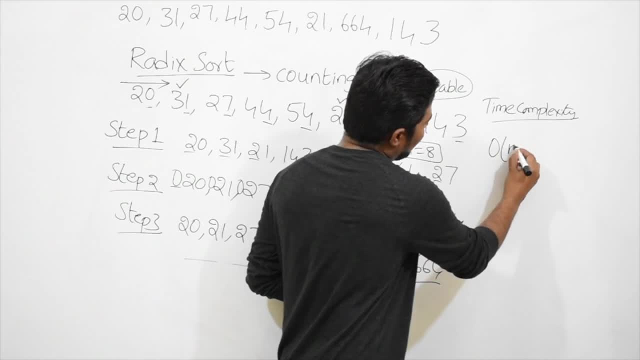 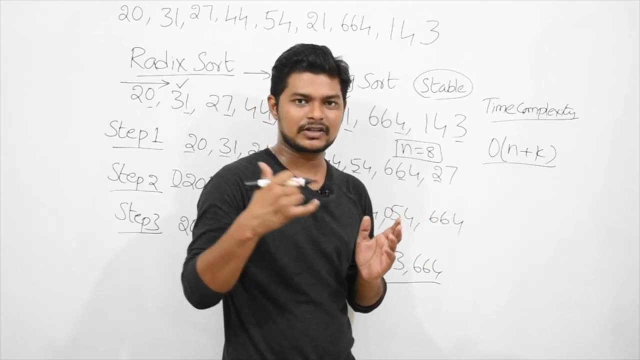 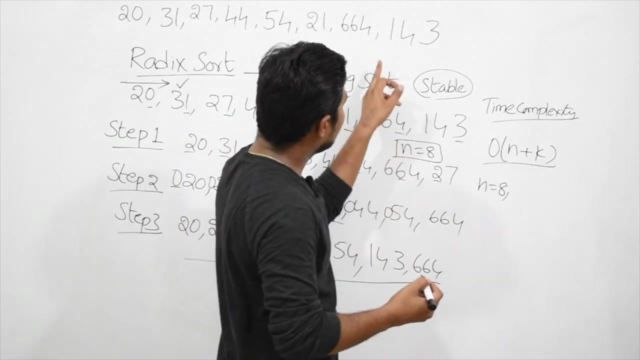 problem. generally for the counting sort it will take we go off n plus K, where K is the range of numbers, since it is derived from the counting sort, like we use counting sort for sorting radix sort. here the total numbers we have taken, n equal to 8 and the number of digits with which we can maximum represent D equal. 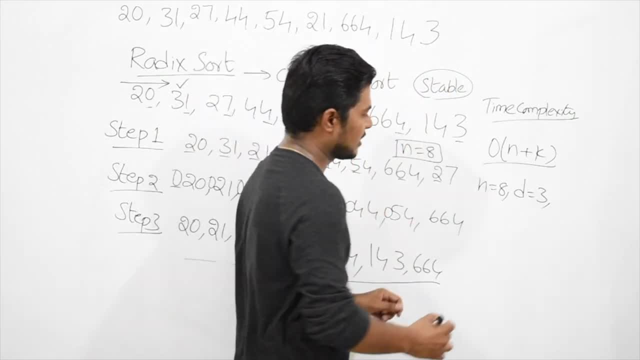 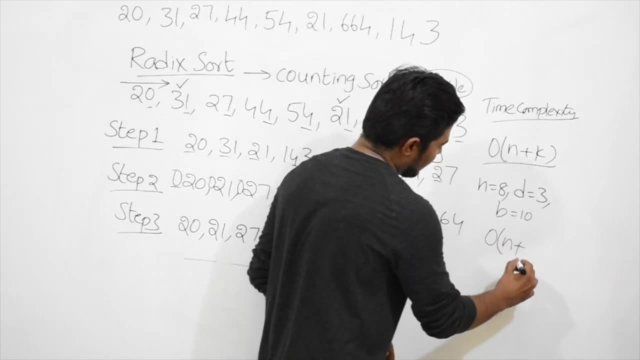 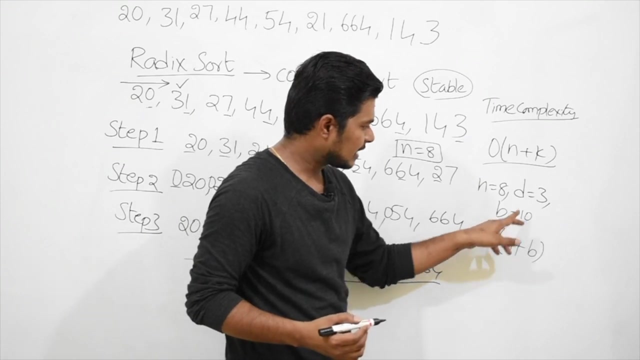 to 3, and here we have taken all in base 10. okay, B equal to 10. so the time complexity can be defined as we go. of n plus P in place of K I have written B, okay now, since here the number of digits also matters in the time complexity we